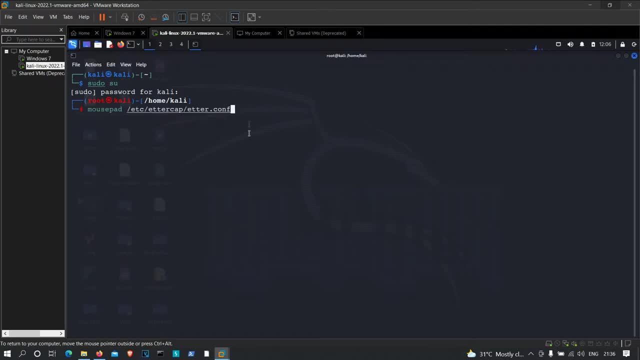 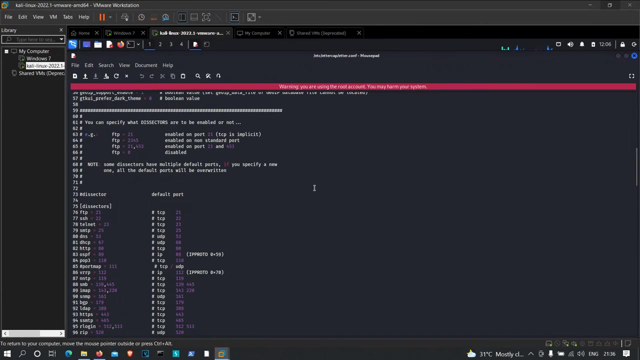 to do is we need to type mousepad And we have to specify the path. So this is the path for iterconf file, which is in the etc. itercap and the iterconf file. So we need to modify this. So what I'm going to do is I'm going to hit enter. And now what we need to do? 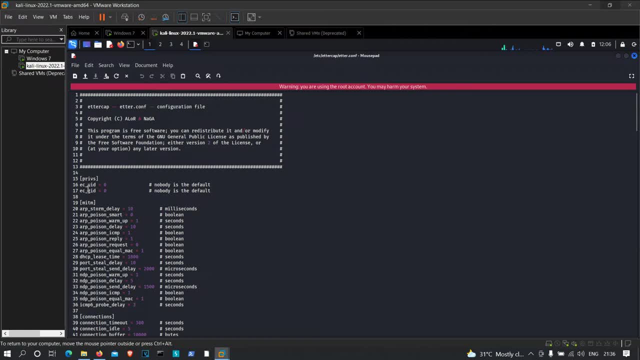 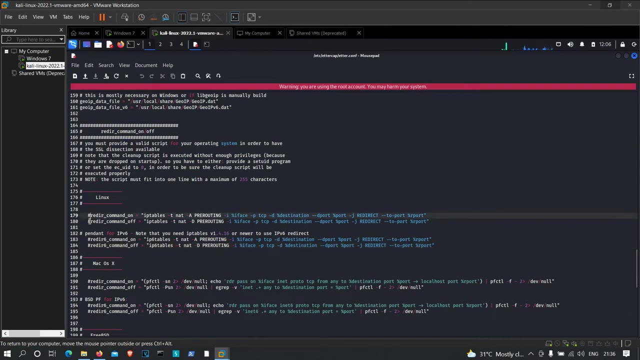 is, we need to modify two things over here. The first thing is that we need to modify this hc__uid and hc__gid to zero, And after that what we need to do, we need to go all the way to the bottom, And here we have to remove this hash from the, from the Linux category. 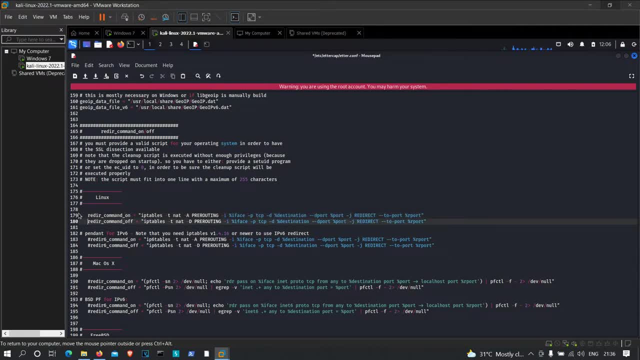 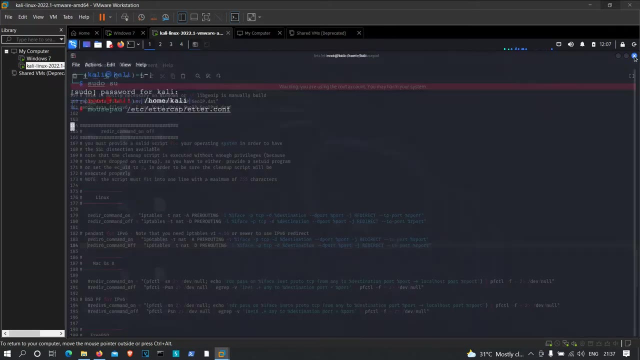 So what we need to do is we need to remove this, And we have to remove this hash from here as well, And all we need to do is just we need to save this file. Now we are done. Now let me close this file, And now let us try to modify the other file, which is the. 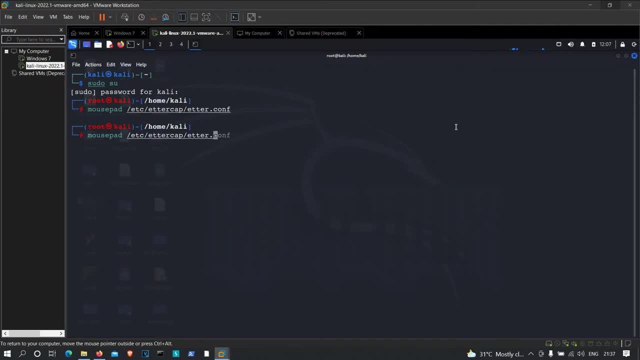 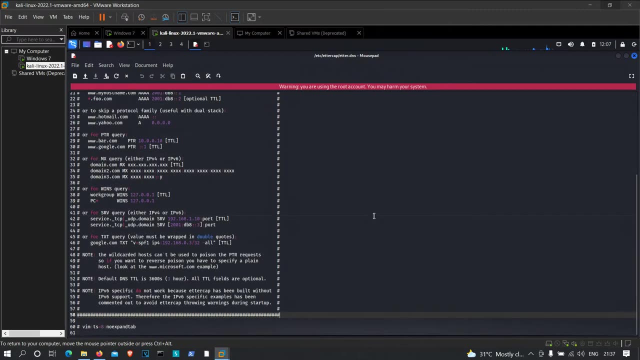 iterdns file. So I'm going to just remove conf from here and type DNS. So this is the file that is going to handle the DNS records for us. So let's say, suppose I want to do something like whenever someone tries to visit the practicaltech, so they will be redirected. 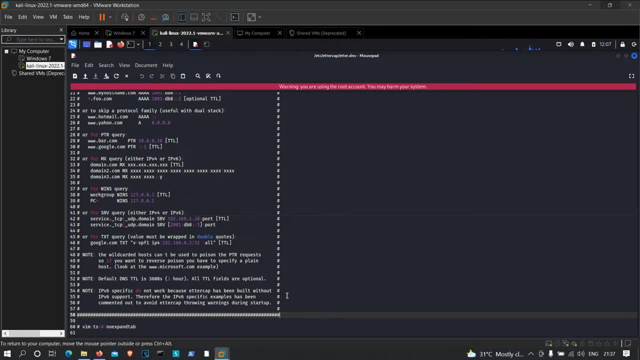 to my own hosted website. So what we need to do in this case is that we have to. first of all, let me add an extra hash over here. Let me get rid of this three, And inside this I'm going to type the domain. 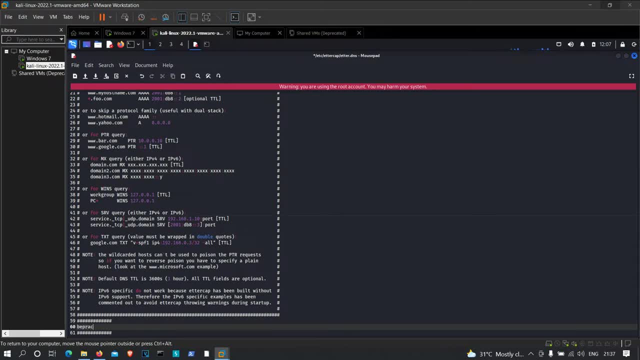 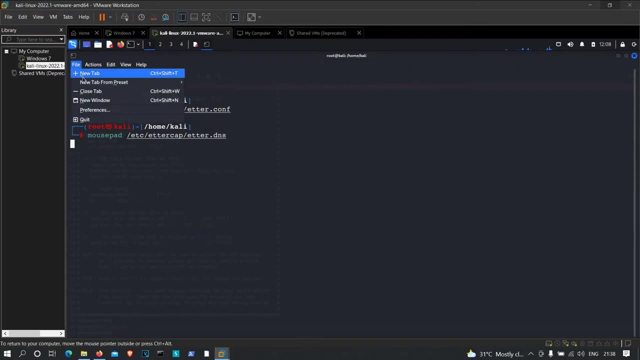 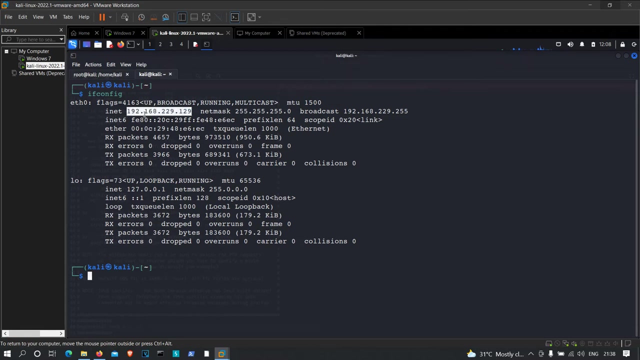 name which I want to spoof. So here it is: be practicaltech, right And now space, and we have to type A, which is for A records, And after that we need to type our IP address. So we can just go Over here and we can type ifconfig And, as you can see, this is my IP address And I'm 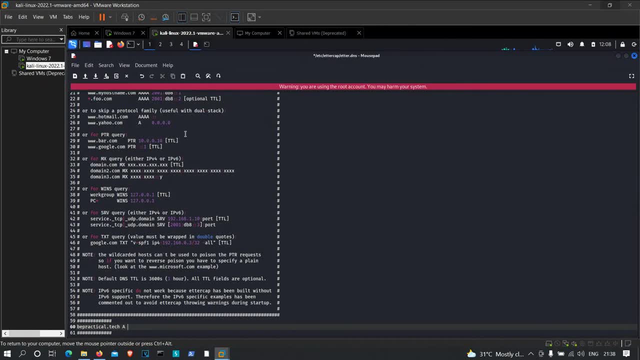 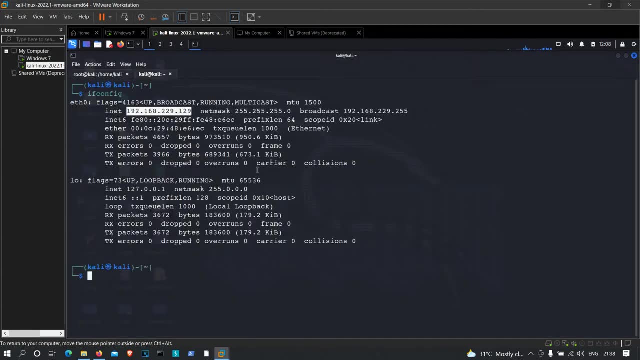 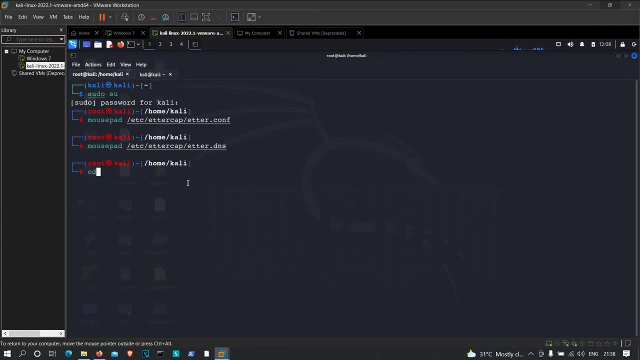 going to copy this And I'm going to paste it over here. Perfect, And now we are done in configuring both of this file. Now what we need to do is that we need to start our own Apache two server. So before, for before that, I'm going to do something like this: 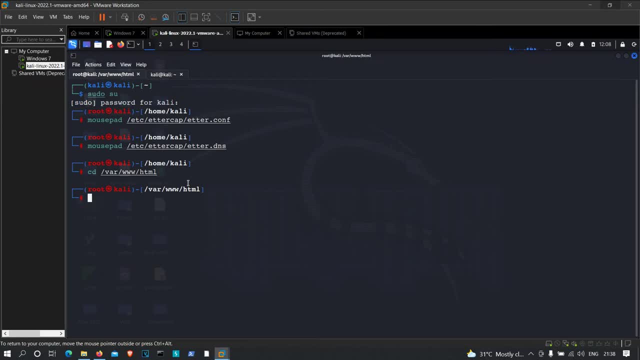 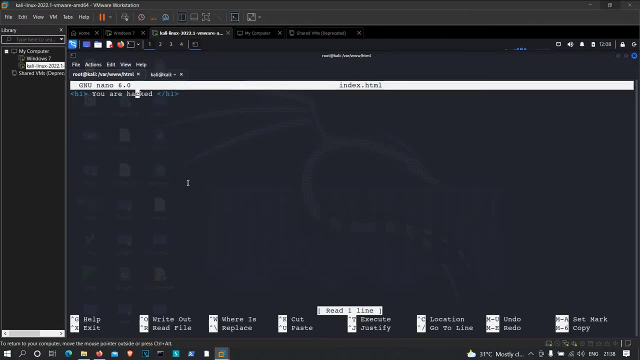 I'm going to visit to my HTML folder section, Okay, And here I'm going to modify my index dot HTML. So, let's say, whenever someone tried to visit be practical dot tech, I'm going to show them that, hey, I own this website. 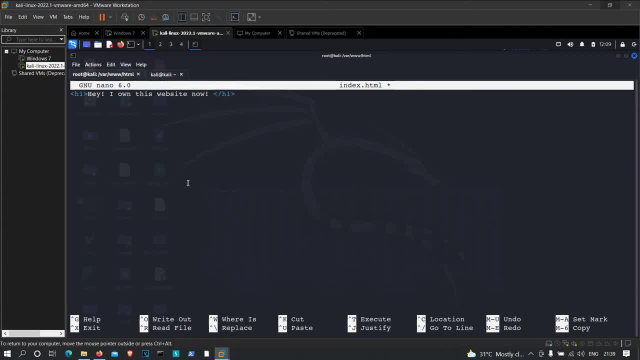 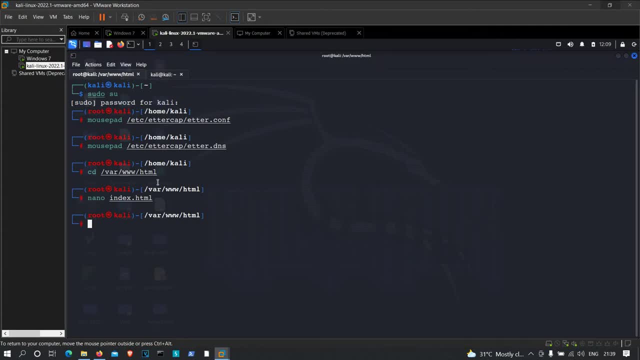 now Okay, and I'm going to save this. So whenever someone tries to visit- be practical tech- the DNS will point to my local IP address, the IP address of the attacker, and here we are hosting our Apache 2 server. so the victim will see: hey, I own. 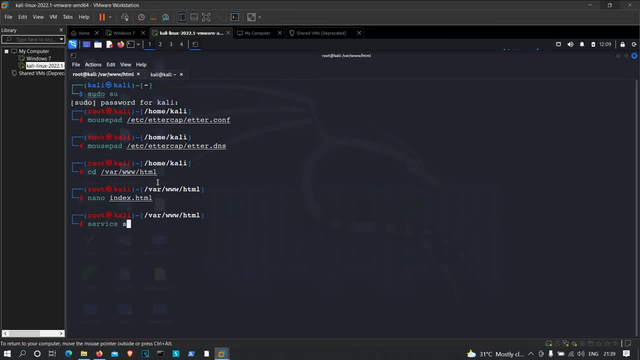 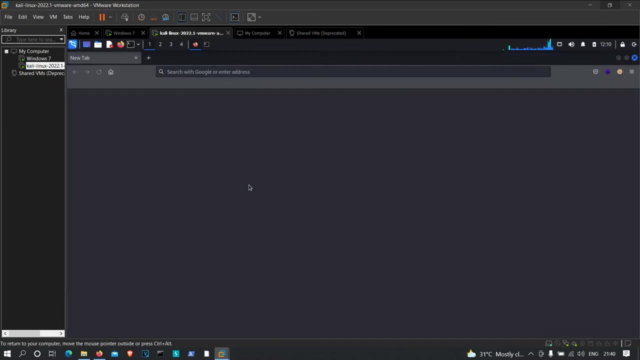 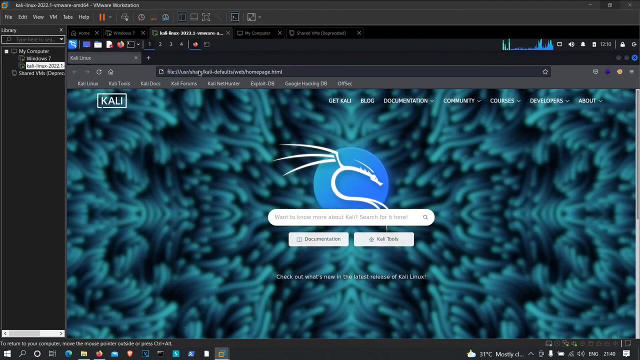 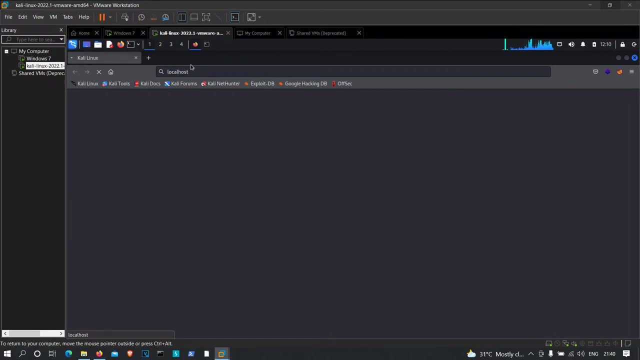 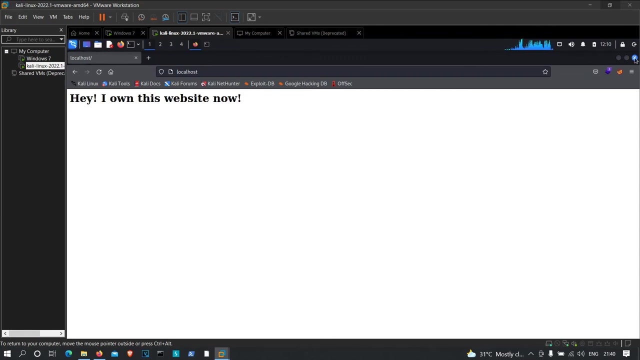 this website now. okay, so let me start my Apache 2 server. Apache 2 start and let us verify whether the Apache 2 server is working or not. and now let me type localhost over here and perfect. as you can see, the Apache 2 server is running fine. now let's head back to the victims machine. 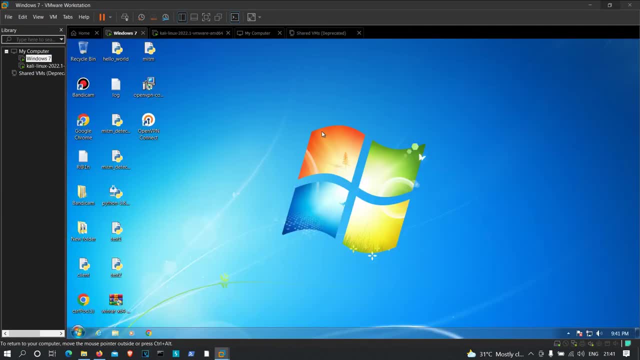 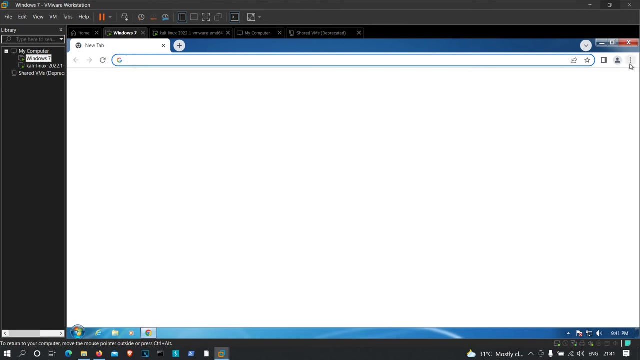 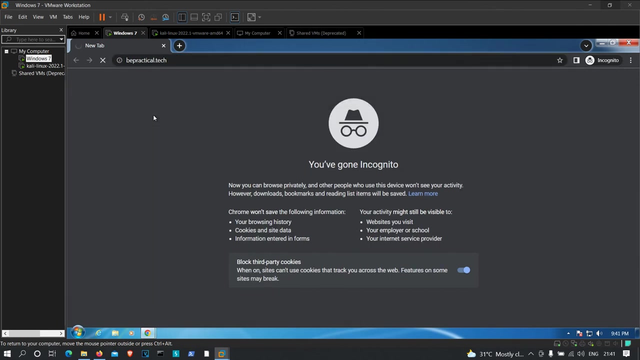 so. so this is the victim machine, and here we are going to see what is the content of be practical or tech before any attack. so let me go to the incognito mode and I'm going to type be practical dot tech. let's see the content of it. 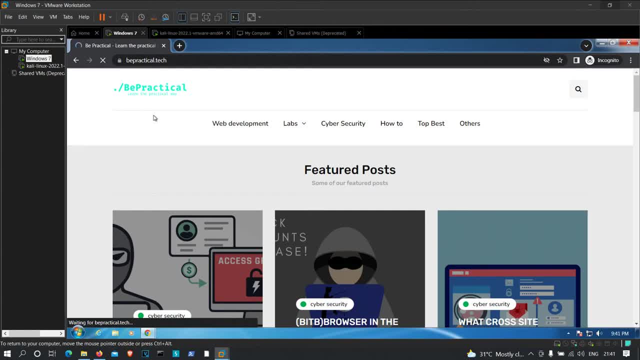 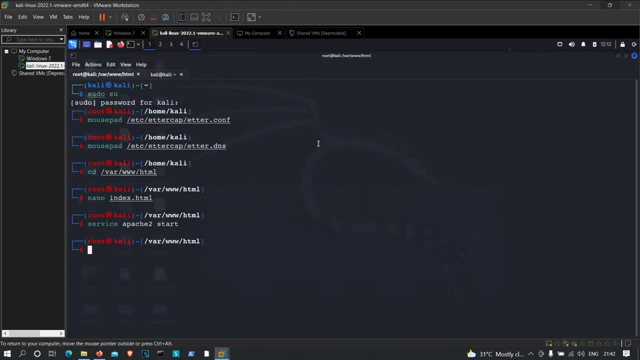 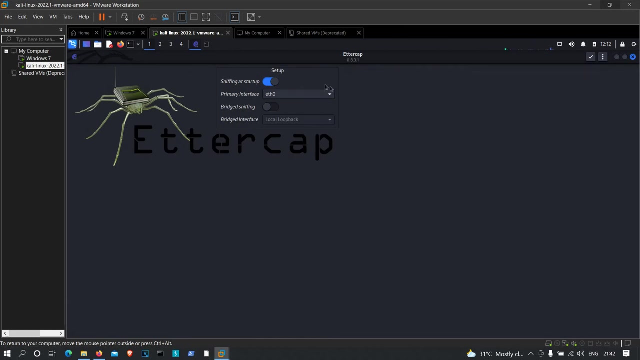 and, as you can see, we get the be practical tech default content on this particular be practicals web server right. and now let's see what happens in when we try to perform DNS spoofing attack on this particular network. So over here we have to type itercap-g, which stands for graphical, and now we have to click.